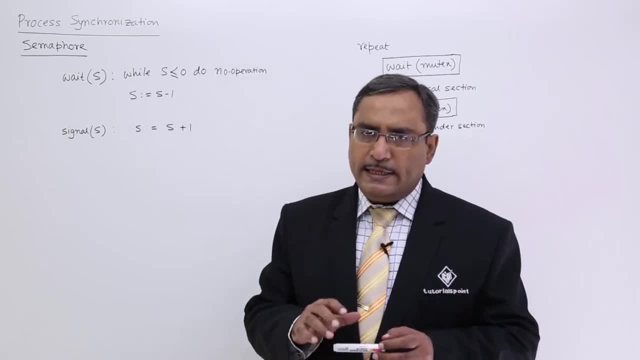 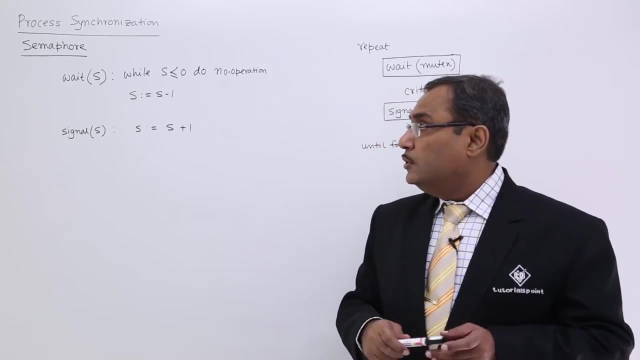 not be executed. Partial execution will not be there. Either they will be executed totally or not at all. If you are not clear with this particular statement, let us discuss this particular one. So wait and signal. they are nothing but some operations on this Semaphore. 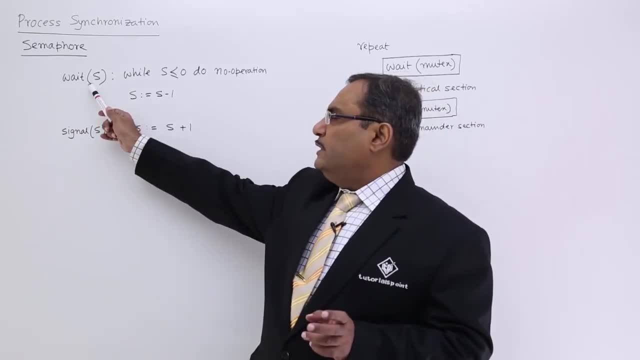 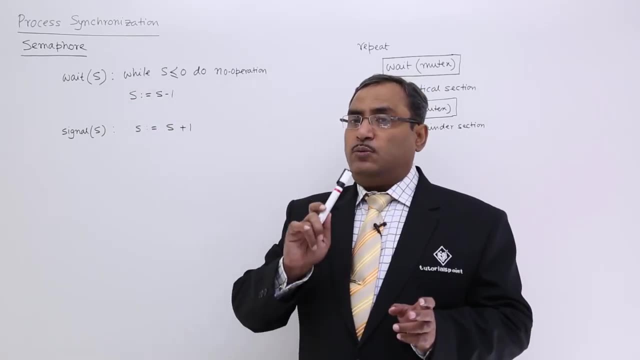 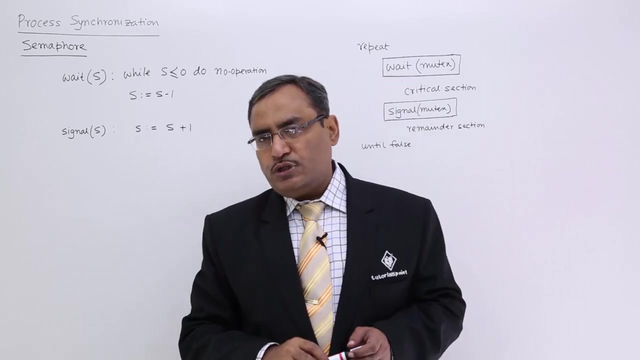 variable, Let it be S, S. So say on this: in this wait I am having statements like this: So if I tell that wait is operation is occurring on the Semaphore variable S, then all these codes will get executed. partial execution of this code is not possible. So that is why this wait and 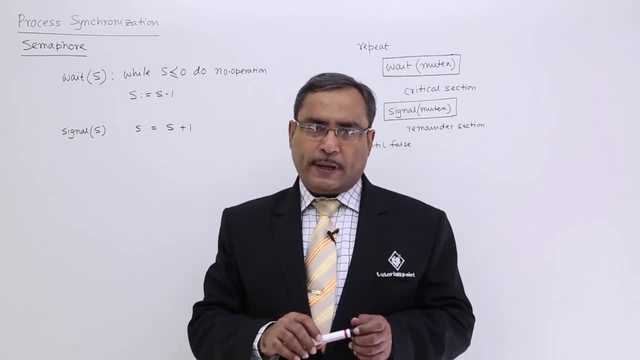 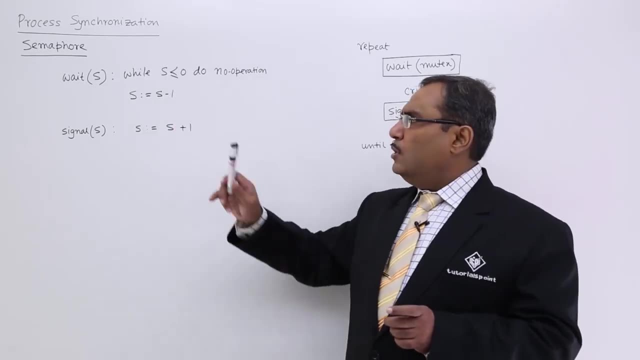 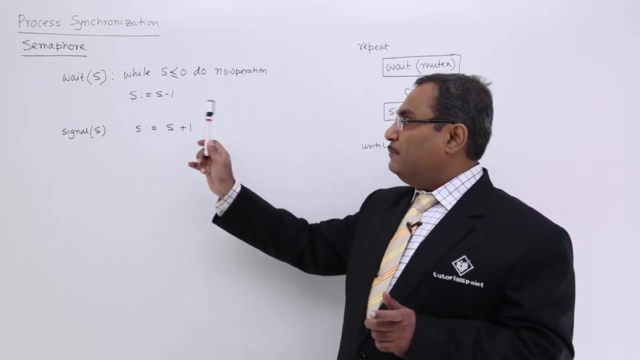 signal should be called as an atomic operation. Now, what is the purpose of wait? It is telling that if the Semaphore value is 0 or less than 0, while S is less than 0, then that is a less than equal to 0. do no operation. It is while it is not. if that means until this. 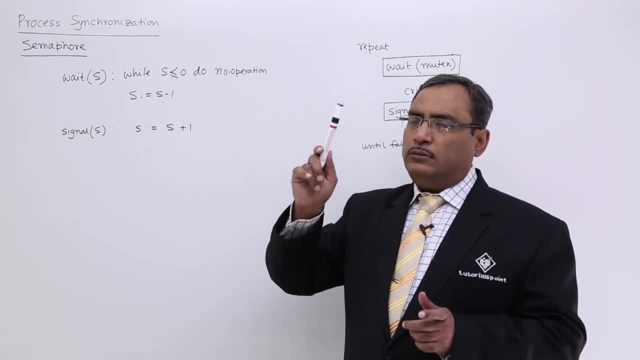 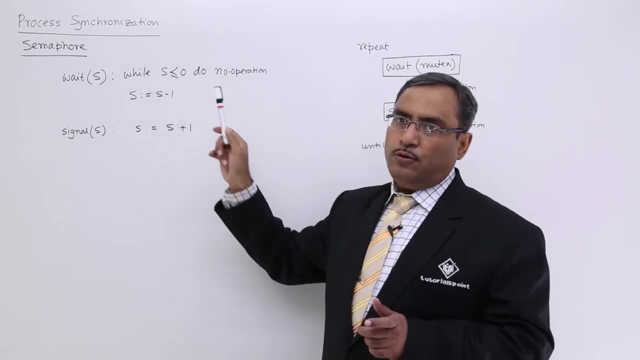 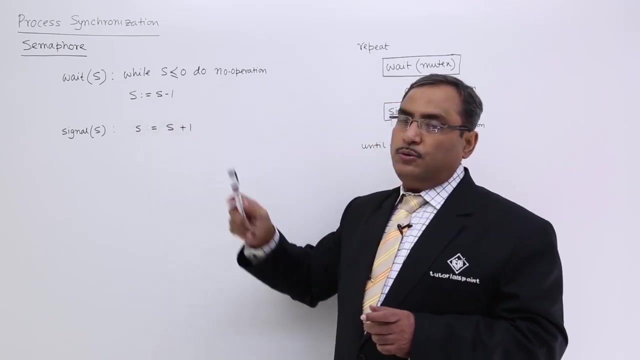 s is becoming not equal to 0 or more than 0. until it is becoming that this, no operation will take place. that means it will go for an infinite loop. When s will be positive and non-zero, then only it will come to the next line which will make s is equal to s. 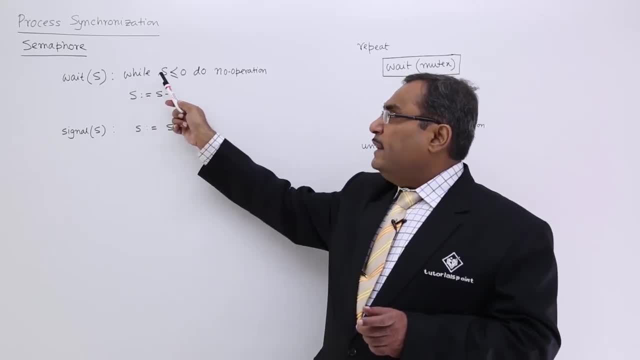 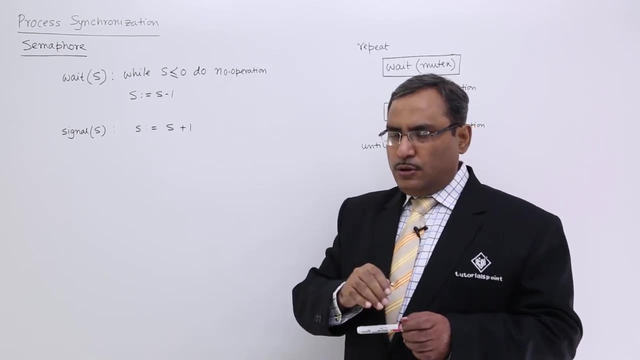 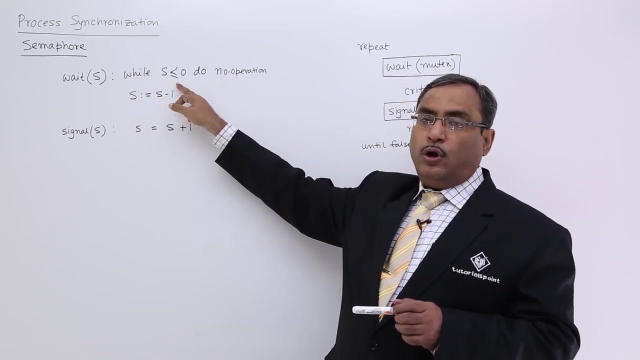 minus 1.. Let me explain it again: while s is less than equal to 0, do no operation. that means whenever the value of s is 0 or less than 0, when it will remain that it will go for doing this infinite looping until and unless s is becoming non-zero, positive And. 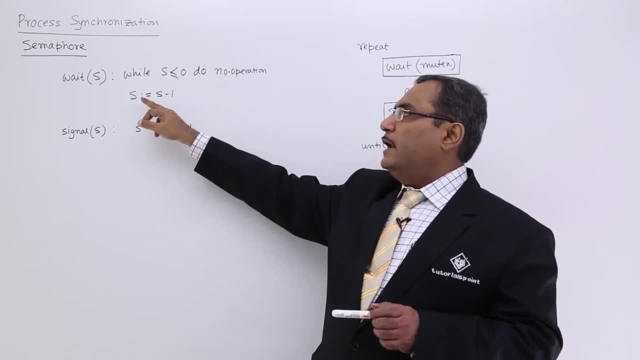 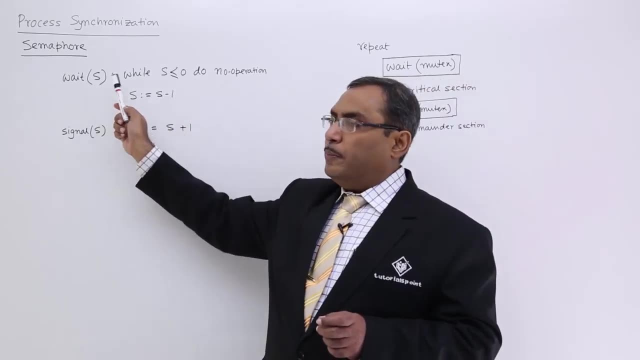 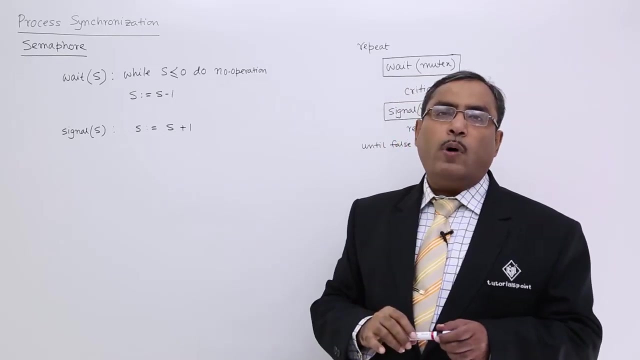 when it is becoming non-zero positive. then it is coming here, and s is equal to s minus 1 will be the next instruction to be executed on the semaphore variable s in this weight operation, In the signal operation. a very simple statement: it will just increment the value of s by 1.. 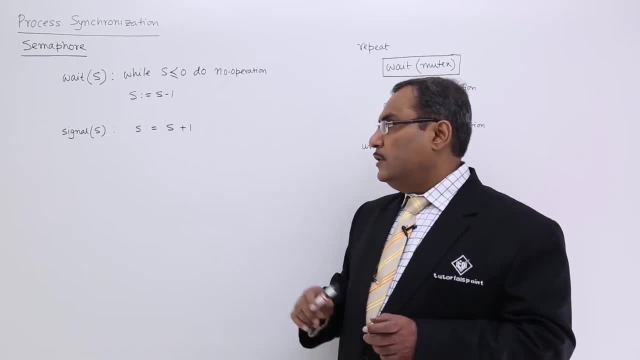 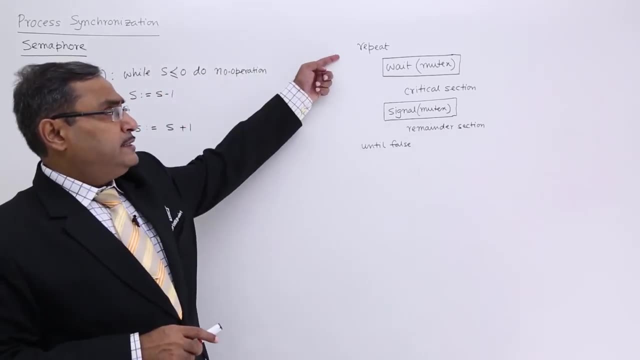 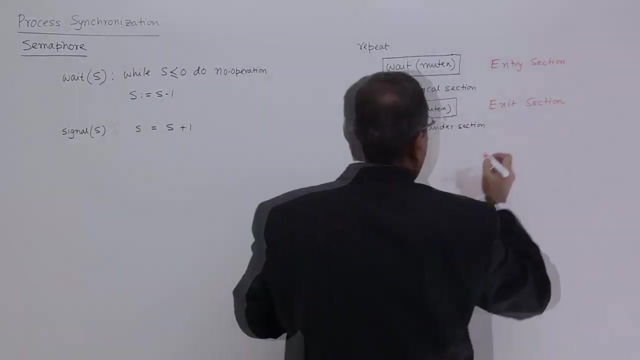 So these two are the atomic operations we are having. you might be asking me what is the use of that. I am just discussing that one with some example Before that. this is the code which we have written in the previous, in the previous example here we wrote in the 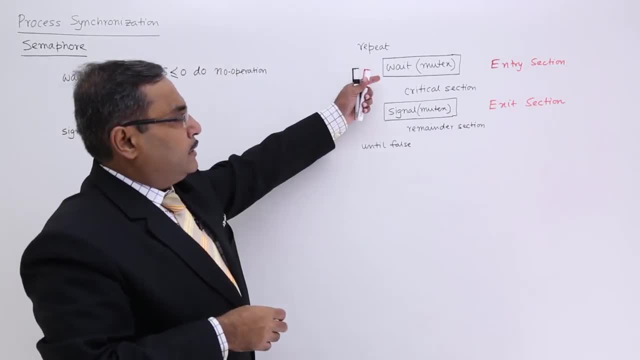 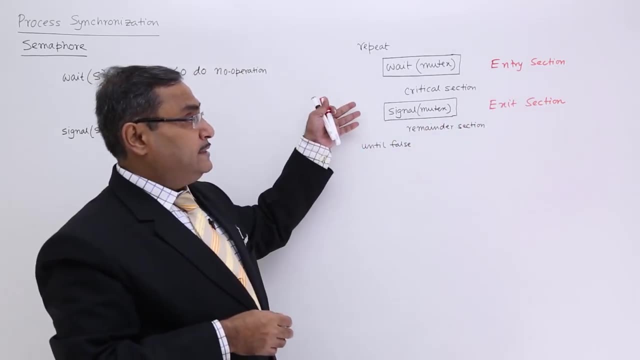 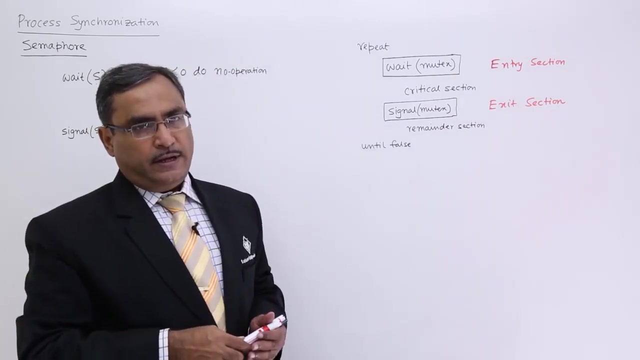 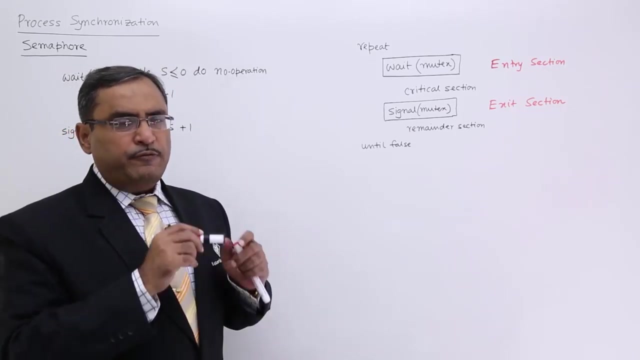 previous section. here we wrote that a weight was So there as entry section and signal was there as exit section, but that weight and signal, these two atomic operations, have replaced this entry section and exit section respectively. So let me explain it further. Let us suppose initially, that is one semaphore variable which 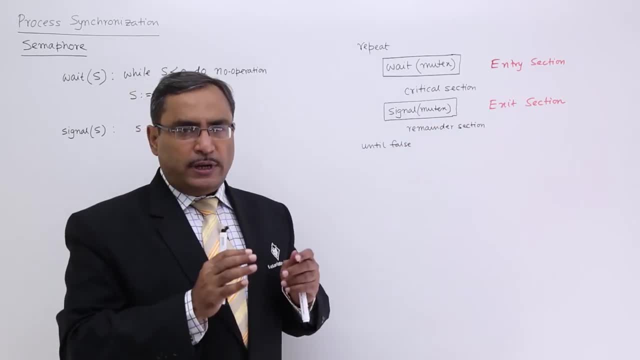 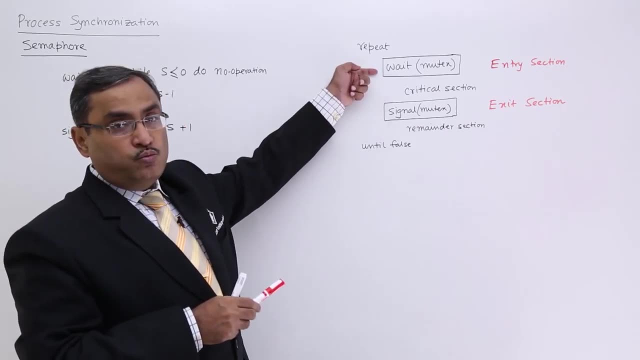 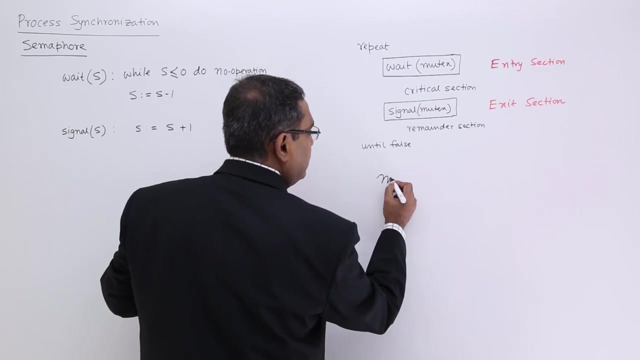 is mutex actually? it is a short form of mutual exclusion. Let us suppose a process can enter into this critical section, When the weight is, when the weight will have its completion, not following an infinite loop. Let us suppose initially mutex is equal to 0. so what is a mutex? it is nothing but one. 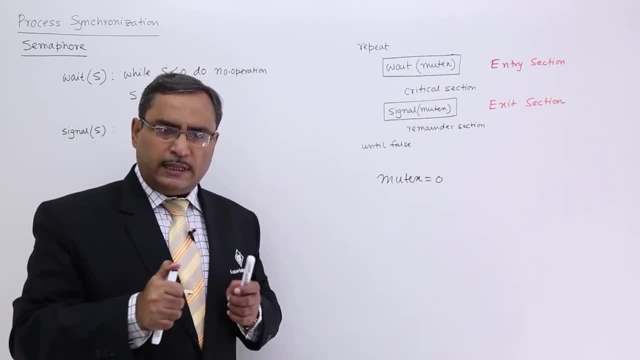 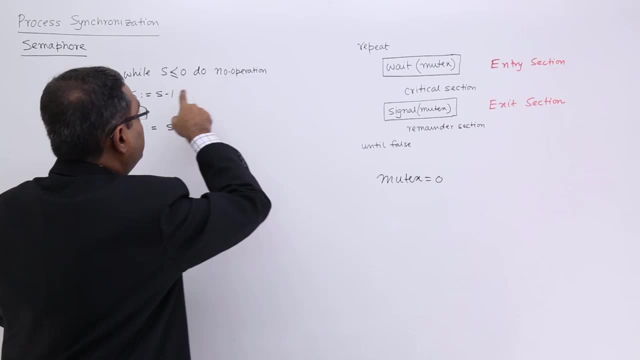 semaphore variable. and if I told you that this semaphore variable is nothing but one integer quantity? So mutex is equal to 0.. So when mutex is equal to 0, in case of weight, it is executing this code, While mutex is less than equal to 0. 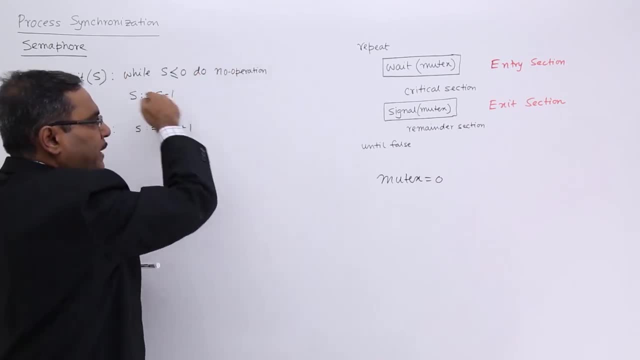 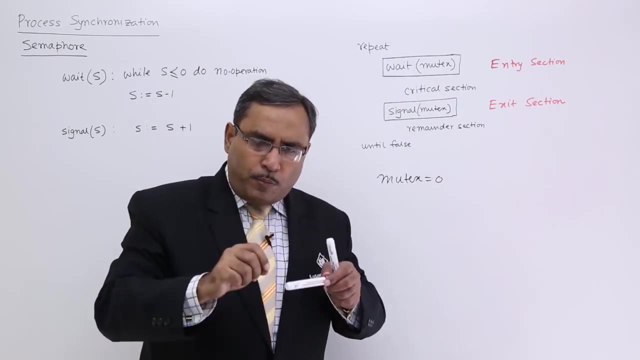 the condition is true, do no operation. so it will go on looping in this way. so the process cannot entered into the critical section. let us suppose at that time the critical section was occupied by another process, let it be p2. so when that process will completes its 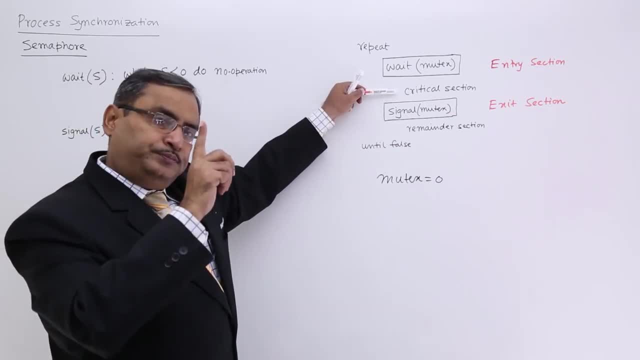 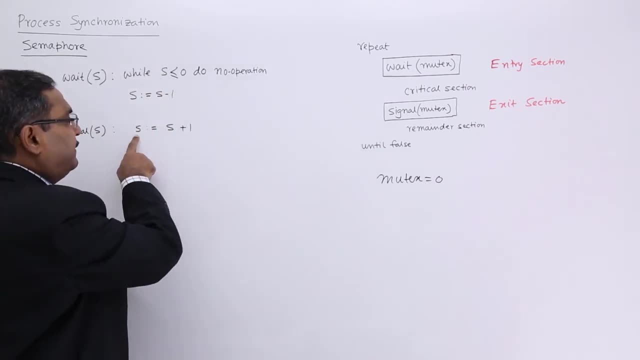 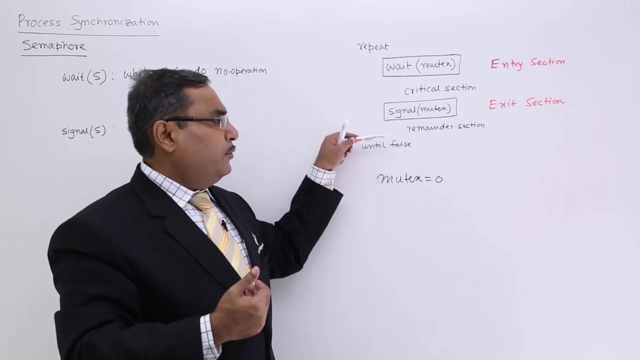 execution in the critical section. when that process p2 will come out from the critical section, then it will execute signal mutex. so in that case the mutex value will get incremented by 1. so when it will leave or exit from the critical section and when it will find itself, 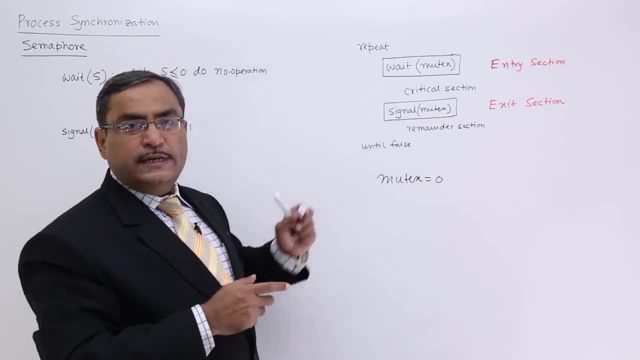 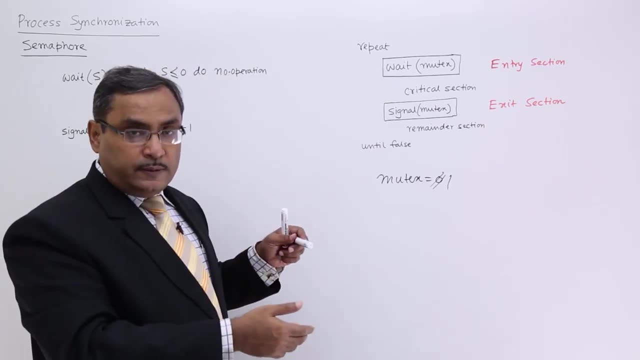 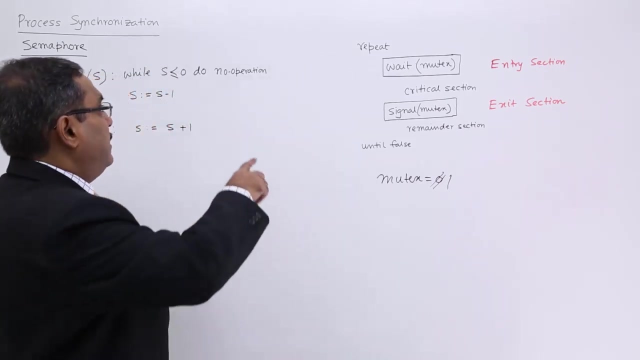 in the remainder section, that process p2, it will make mutex is equal to 1 and it will make mutex is equal to 1. so, as a result of that, what will happen? as a result of that, that the next process which which i was discussing, let it be p1 which was waiting at mutex, because 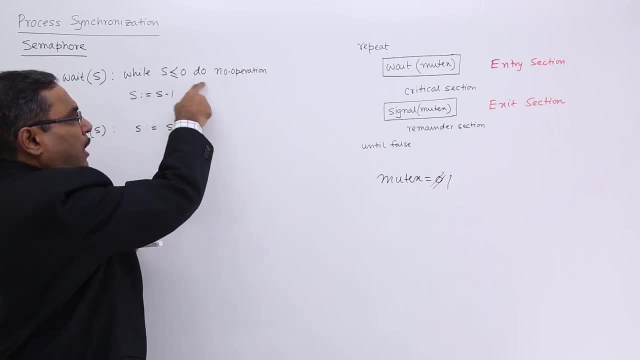 this particular s. at that time mutex was 0.. So now the mutex has value 0. So this condition will become false. so it will come out from the from this: while body and then the mutex is equal to mutex minus 1, will get executed. 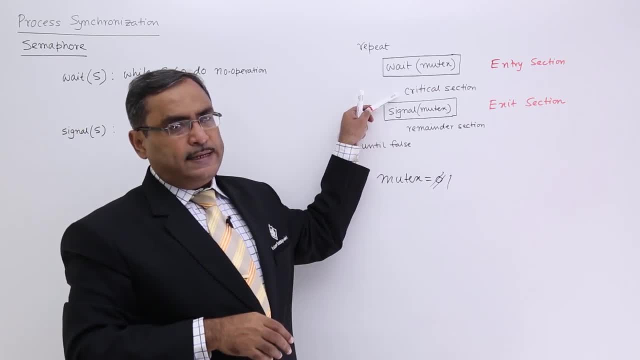 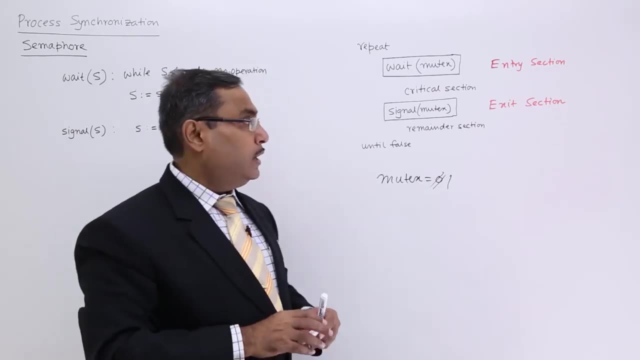 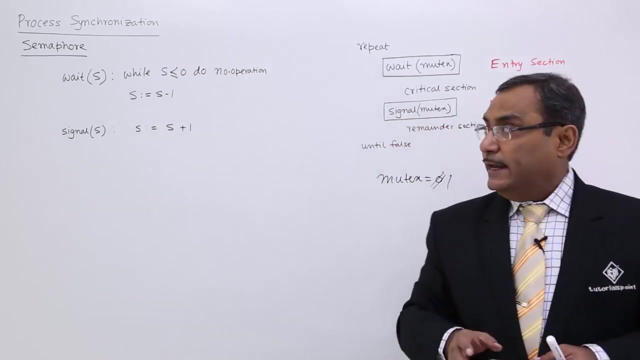 So now it will come into the critical section. the process will have its execution again when it will be leaving. the p1 will be leaving. p1 will again, again make mutex is equal to mutex plus 1 in the operation signal mutex. So what will happen? another process can go and entry into the critical section in this. 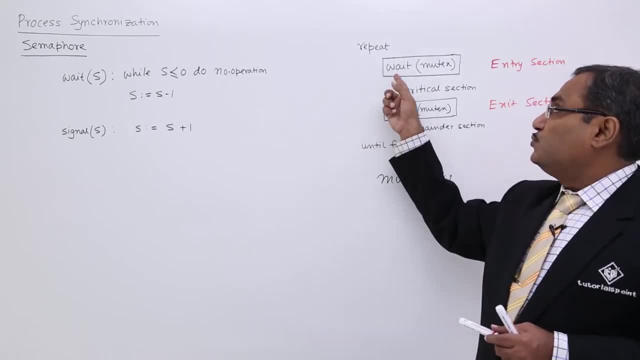 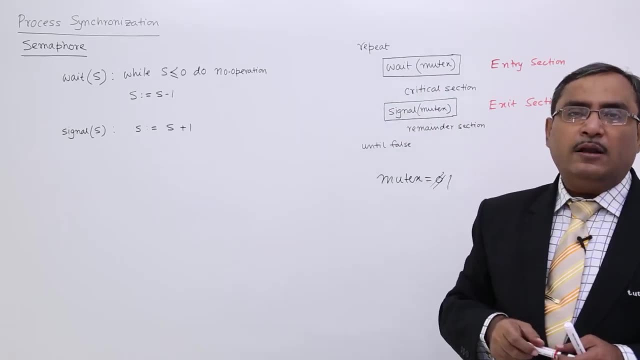 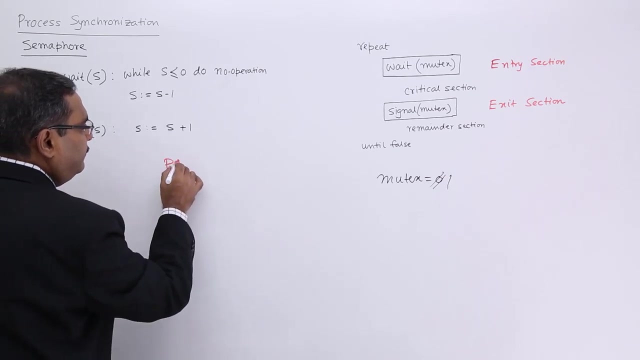 way. you see the previous diagram, I have updated this one. So entry section has been updated by wet mutex and this exit section has been updated by signal mutex. So let us go for another very small example. Let us suppose we are having one process, say p1, and say another process, say p2.. 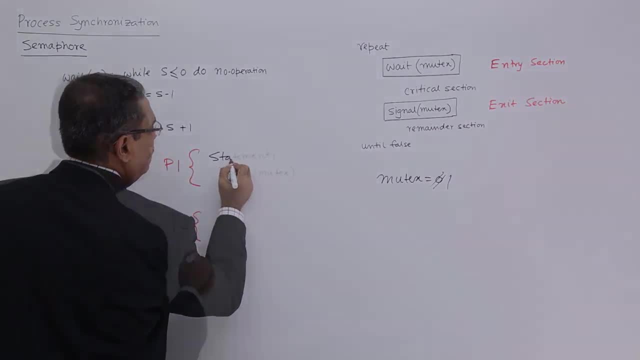 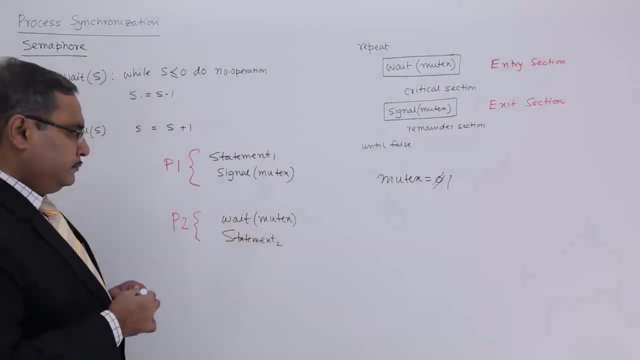 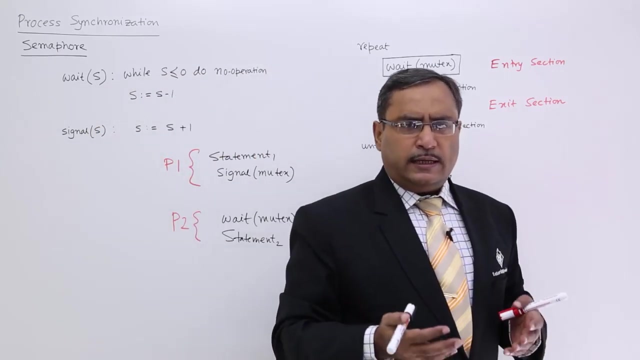 This p1 is having a code like statement 1.. So p1 is having a code like statement 1 and signal mutex, and p2 is having a code like wet mutex and statement 2.. What is mutex? Mutex is nothing but one synchronization variable, mutual exclusion- ok. 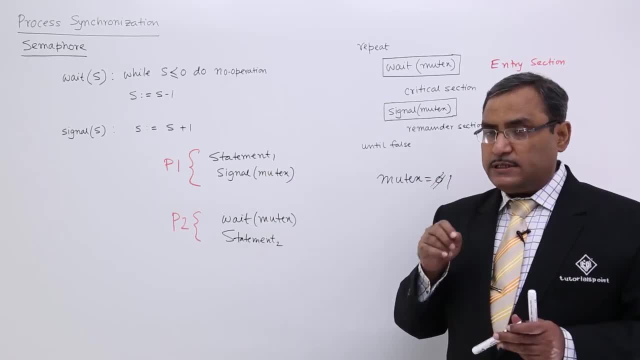 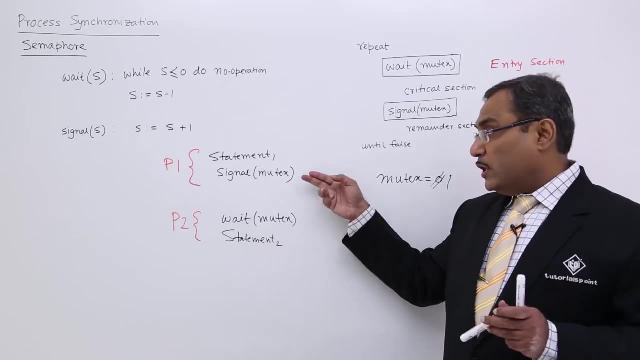 Now I want p1 should execute at first, then p2. let us suppose p1 is the washing process and p2 is the drying process of clothes. So washing process should come at first, then drying process will come. So that is my analogy. ok, 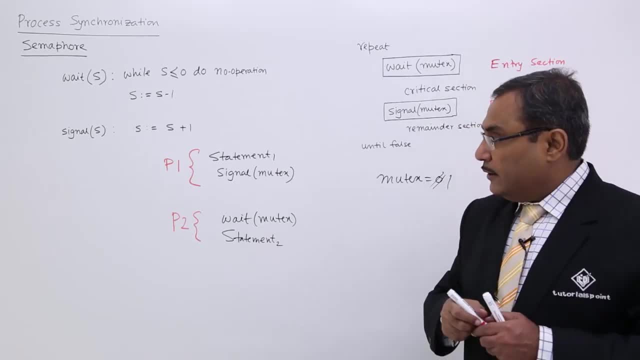 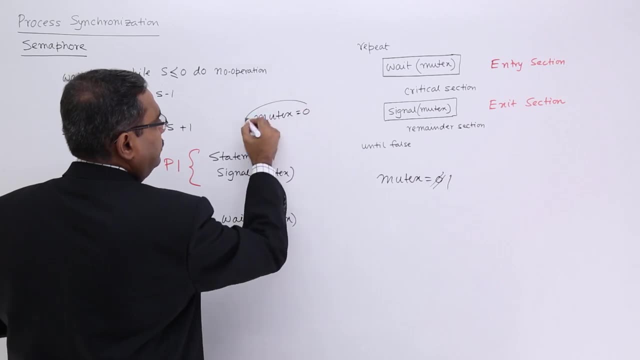 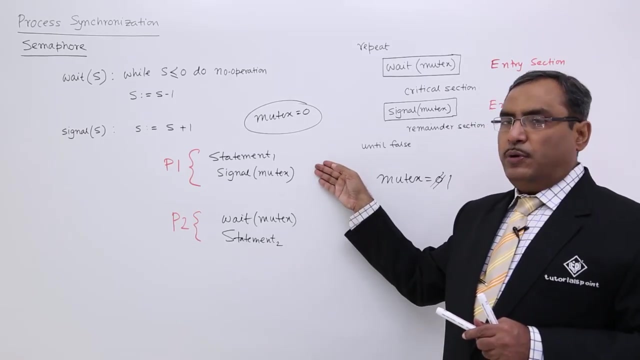 But let us suppose p2 has arrived at first. Ok, Now, another thing is that initially the mutex value is 0. Initially the value of mutex is 0. I was having the recommend to have execution of P 1 earlier than P 2.. Good, Now say mutex. 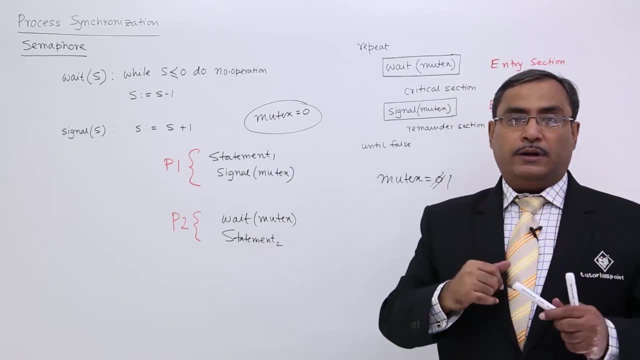 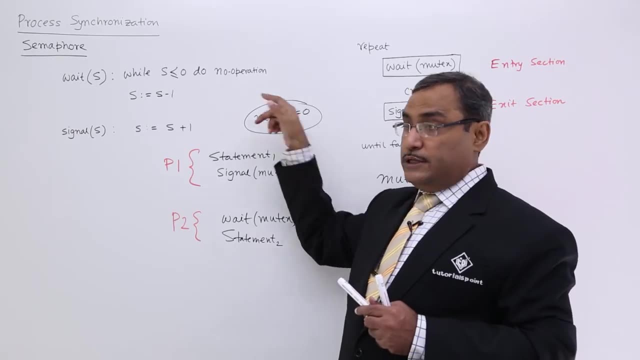 is equal to 0 and P 2 has arrived before P 1.. Then P 2 is having wait mutex. So now, while mutex is less than equal to 0. So it is true, Do no operation. So this particular 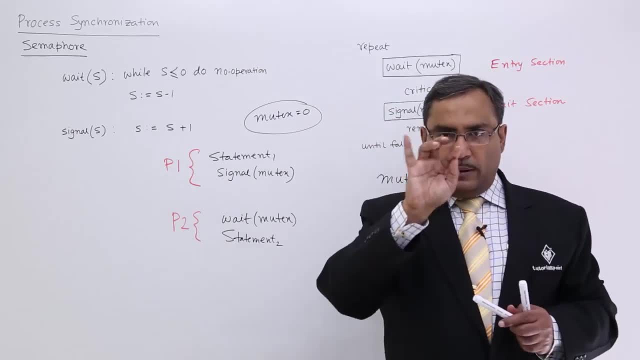 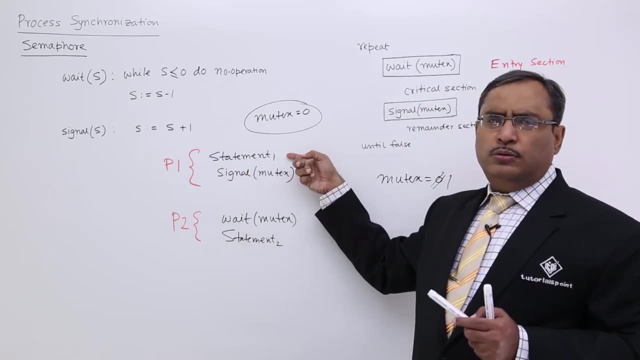 P 2 will get blocked here. It will fall an infinite loop. Why? Because the condition is true while body. So after sometime P 1 has come. So P 1 has nothing to do. before executing statement 1.. So what about the statements written in statement 1? They will.